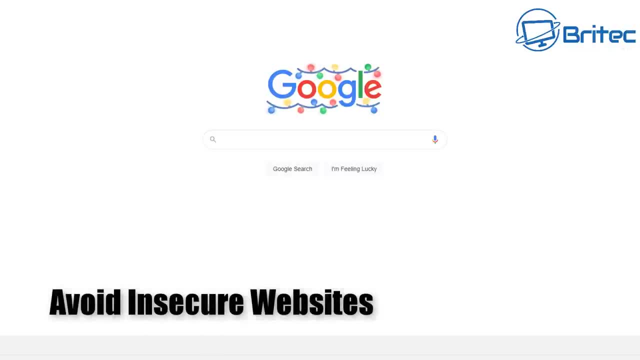 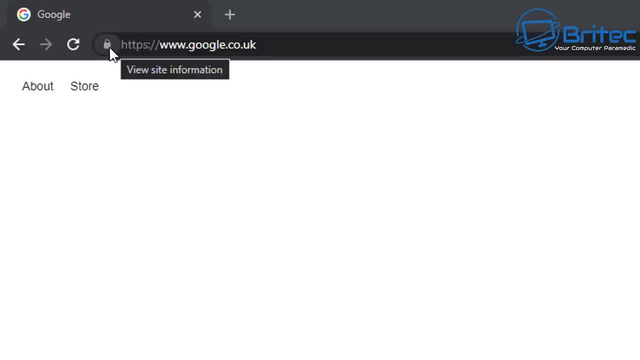 things that you want to make sure that you've got set in place. Next up, we're going to be talking about avoid insecure websites. If you look up the top here on your web browser, on the top left you will see a padlock. If you don't see a padlock here, that means the website is not secure. It's. 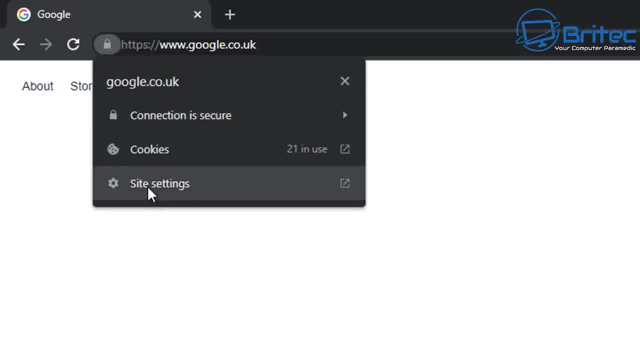 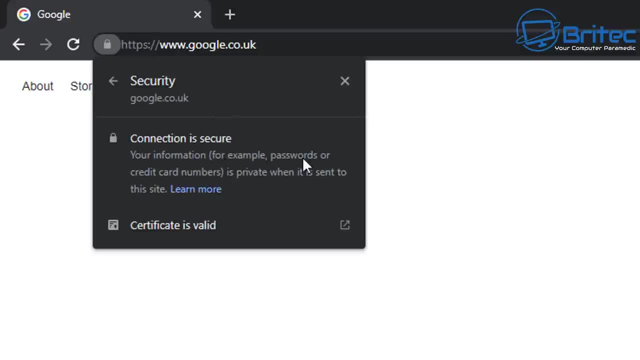 not using HTTPS and you can see that it's not using HTTPS. So if you're on standard protection, you can see here connection is secure and we can see all the information about this. So when you click on here, it will say your information- for example, passwords or credit card numbers- is. 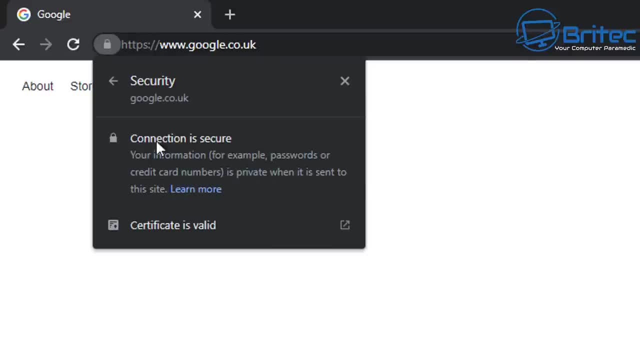 private when this is sent to this site, and this is because it's got a padlock on it, So any sites that don't have this padlock it's not secure. You can see the certificate is also valid, and these are the things that you want to check before you go to any sort of website, especially if you're 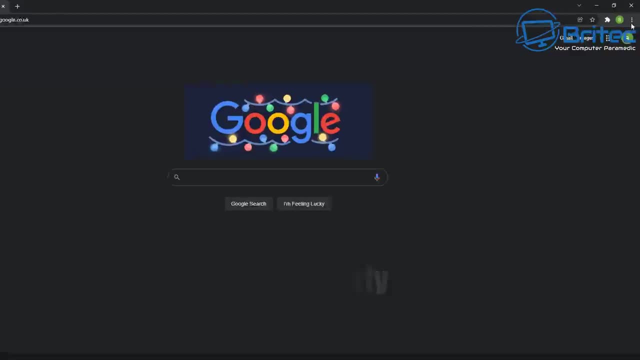 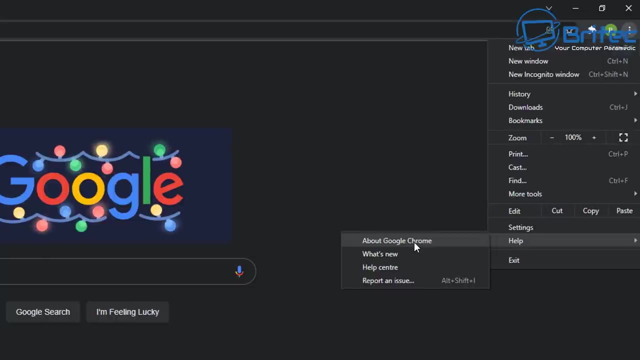 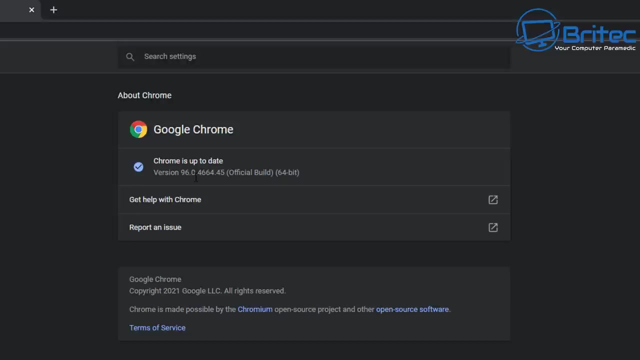 doing some sort of payment on the internet. Now, if you don't have this set to automatically update, then you can be running a outdated browser. It's important that you use the very latest browsers from Google, and this way you will get the most secure browsing experience possible. Now, they normally update this every month or so. 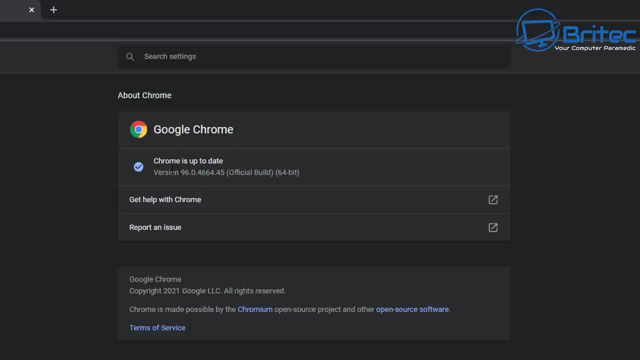 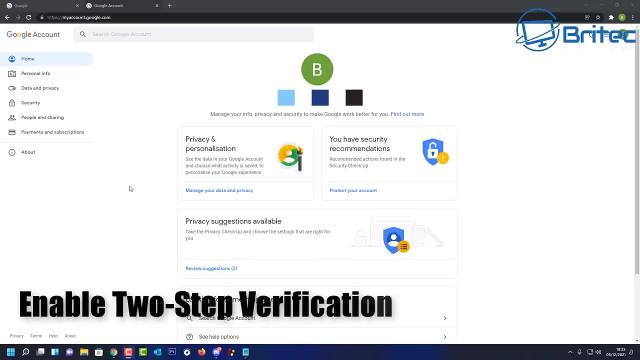 so always keep this updated. You can go in and check manually, but make sure that you have it set to automatic and that way you will be updating your browser in the background Next up, enabling two-step verification. This is something I see a lot of people avoiding because it's too. 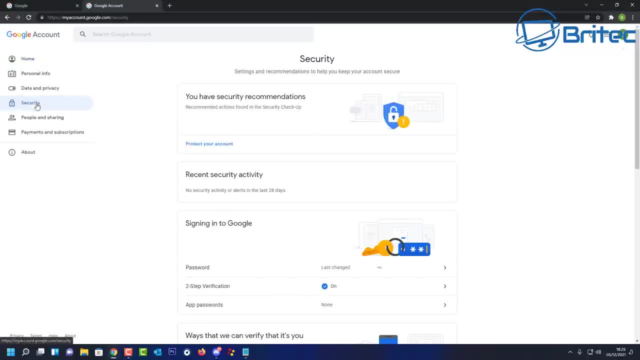 much hassle, but really you should be using this for all of your Google accounts and any other type of account that is really important to you, especially money type accounts. You can see here on the Google account it's set to two-step verification and that should be on and any time. 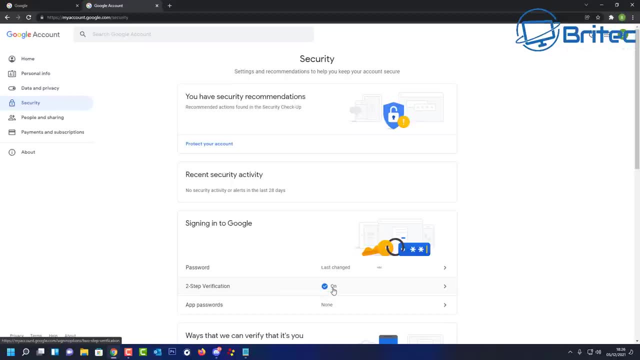 you go to log in. if you log out of your account, it will send you a text message to your mobile phone and it will authorize it. You also want to make sure you change your passwords on a regular basis here, and this means that you're staying very secure and you're 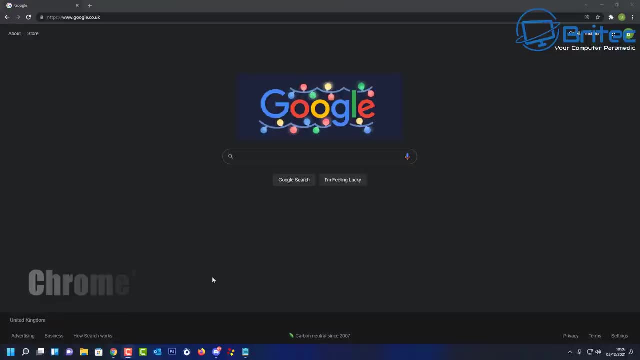 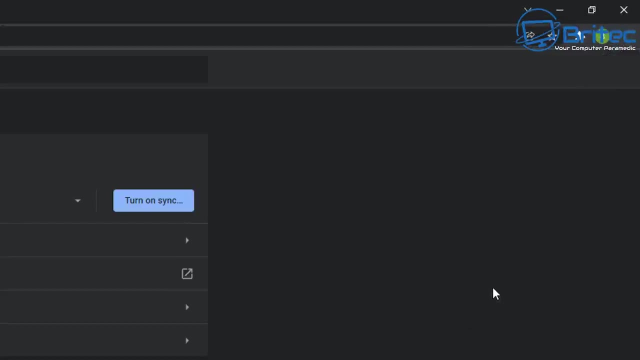 not going to have any sort of security breach on your account. This is important. Next up: Chrome safety check. Always run this Chrome safety check every now and then, just to make sure that you don't have any sort of issues with your browser. Chrome has a built-in tool that allows you to test how. 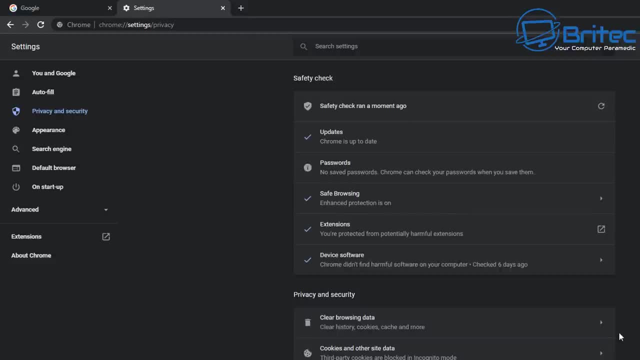 secure your browser is. This tool will also help you identify any data breaches, available browser updates and any sort of malicious extensions that you may have installed on your browser. So it's important that you run this check tool on a regular basis to make sure that you don't have any issues. You can see it will go. 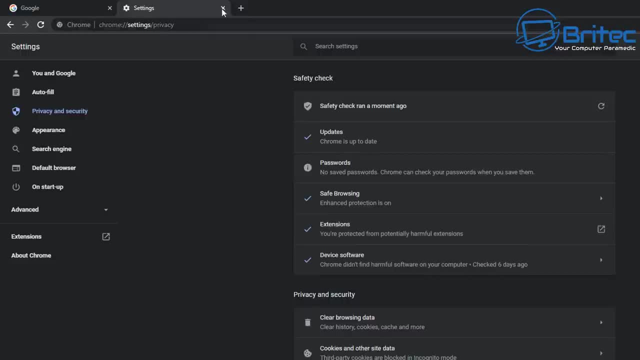 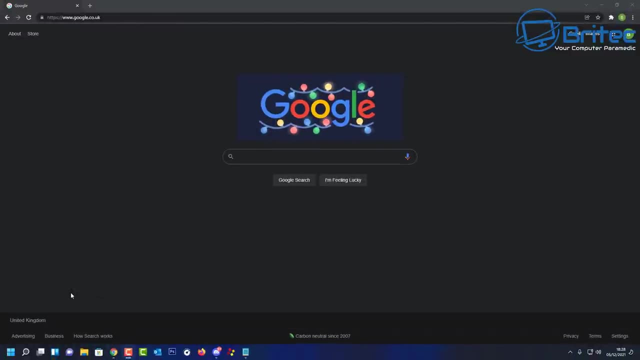 through a bunch of checks like updates, passwords, safe browsing, extensions and other tests like that, to make sure you are safe. Next up, we're taking a look at clean your computer. While antivirus software does the job of removing malware from your system, it can also miss. 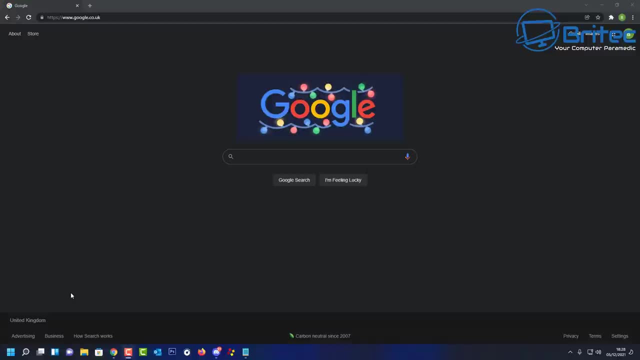 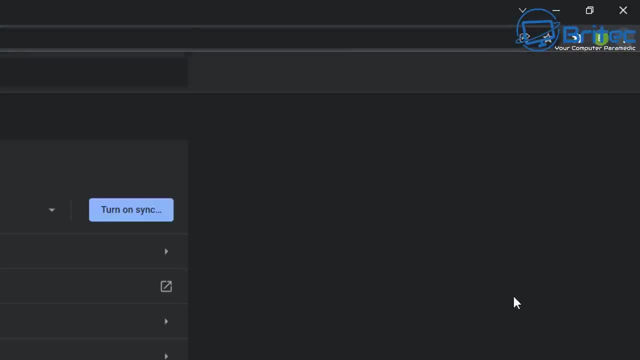 potential threats built into your browser. If you are using your browser, you will need to use a clean up feature that will help you to get the most out of your browser. This is a clean up feature that you can use to get the most out of your 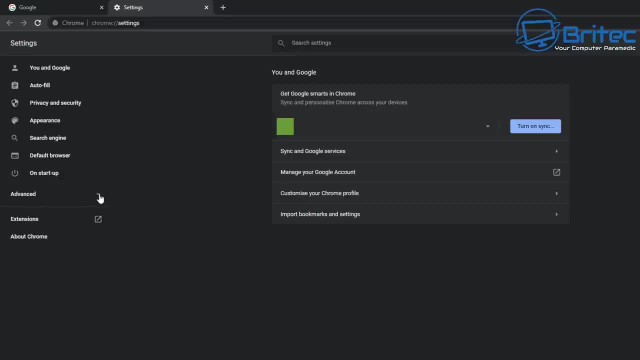 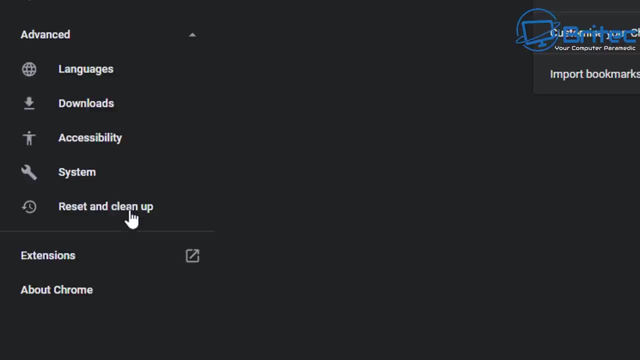 browser. So you'll need to go to your browser and click on the clean up feature and it will show you all the settings that might be hiding, and this could be like man in the middle attacks and things like that. So, going up to the three dots here and going to settings and then inside here, 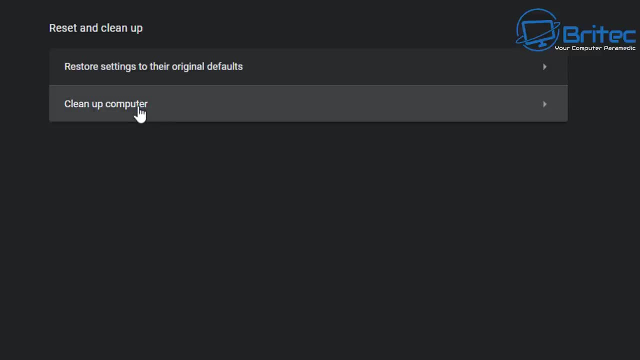 you can go down to the advanced section on the left hand side here. Drop this open and you should see reset and clean up. Hit this clean up computer and this will go through a bunch of checks to make sure that your browser is safe. You can see Google Chrome finds harmful software on your computer and removes it. Report details to: 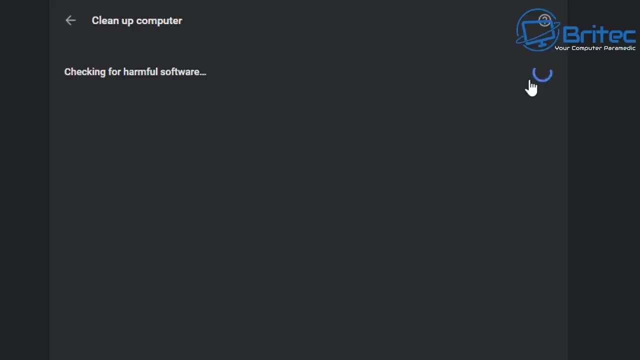 Chrome about harmful software, system settings and processes that were found on your system. This is to help keep your browser nice and safe. Any sort of exploits will be found and detected and then be sent back to Chrome to make sure that these don't infiltrate your system again or any. 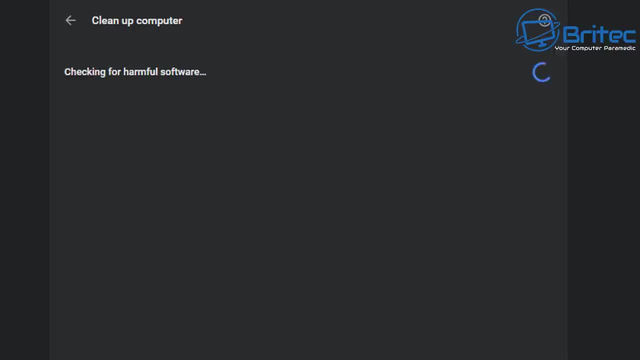 people that are using Google Chrome, So that's a good feature to have. So checking for harmful software will take a bit of time. Let it run its checks Now. it's important that you run other software as well on your computer and do regular maintenance, like virus scans, and also run other 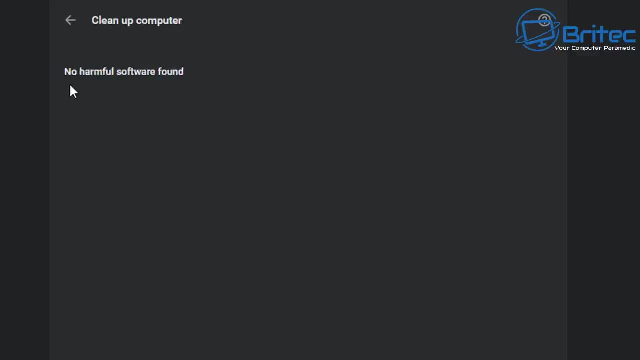 malware scans like Malwarebytes, Hitman Pro and ADWCleaner, which will remove pups and other types of software that's installed on your system. You need to run these, along with these sort of checks as well, just to make sure that your system isn't being breached. 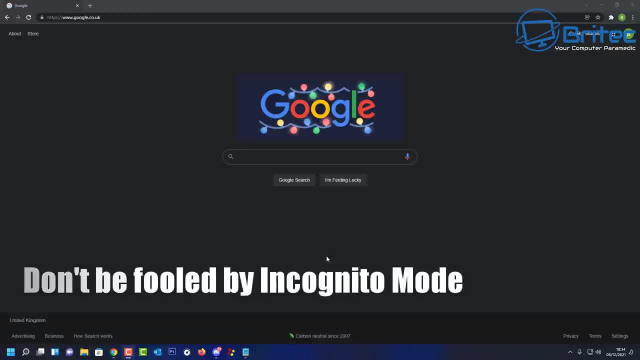 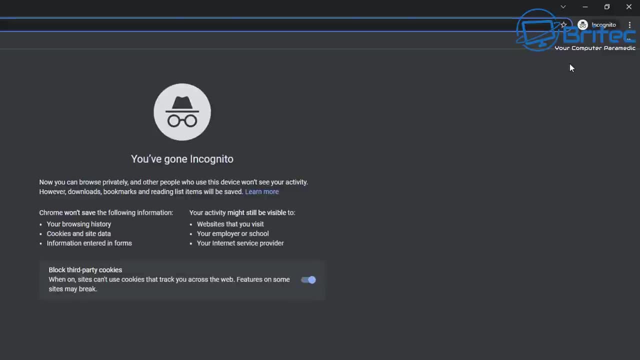 And you have malware built in. If you use Windows Defender, that should do it automatically Next up. don't be fooled by incognito mode. A lot of people fall for this thinking they are completely invisible on the internet when they use incognito mode. But basically you can see here. 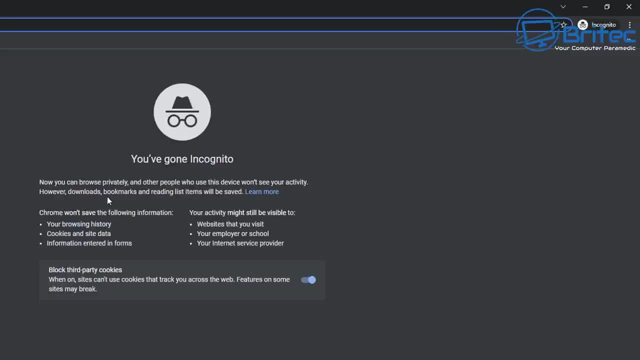 what it's telling you this will actually do. Now you can browse privately and other people who use this device won't see your activity. However, downloads, bookmarks and other reading lists, items will be saved. See here your browsing history, your cookies and other data and information entered in forms will. 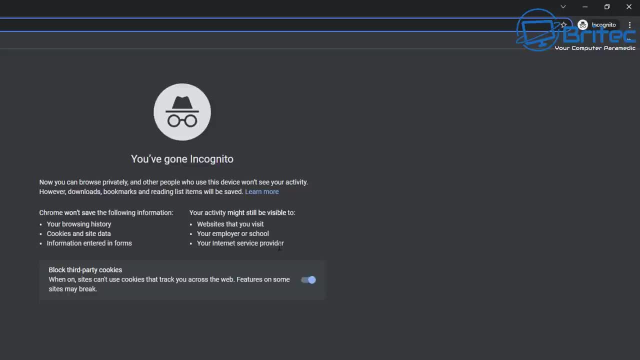 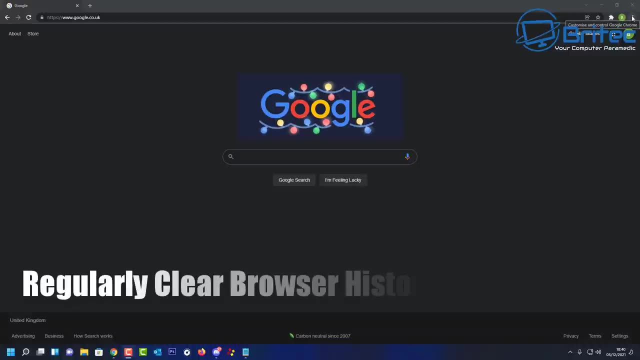 not be saved on your system, but it will save websites that you visit. Your employee or school may be able to detect this, and also the internet service provider, which is your ISP, will be able to detect this. So regularly clean your browsing history as well. This is also another essential. 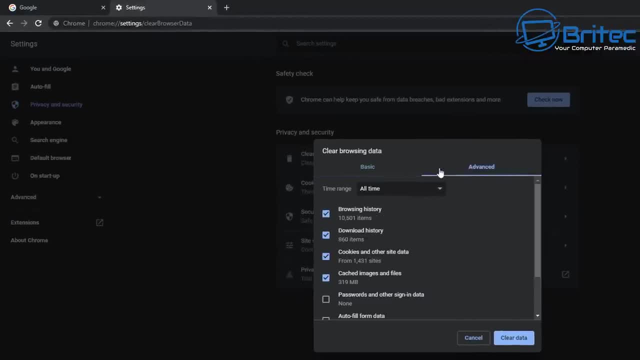 part. You can go into your privacy and settings and clean browsing history. You can do advanced, you can do basic, depending on what you want to do. This will remove all of your browsing history from your computer, depending whether you want to do all time or you want to do just the last hour or 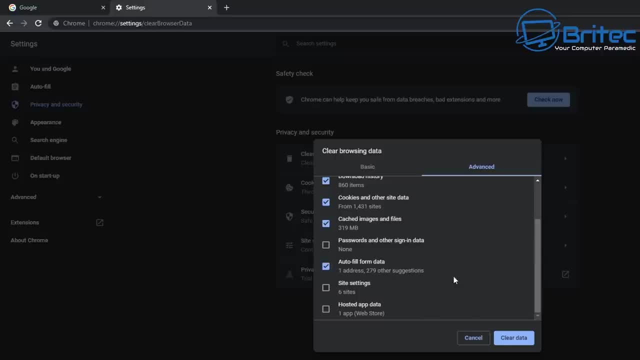 so I'd advise you to do all time and remove all the autofill information, All of the passwords and other signing information and data stored, Cookies and other site data. This will remove passwords as well. So if you're thinking that you've took the tick out of passwords and other signing and 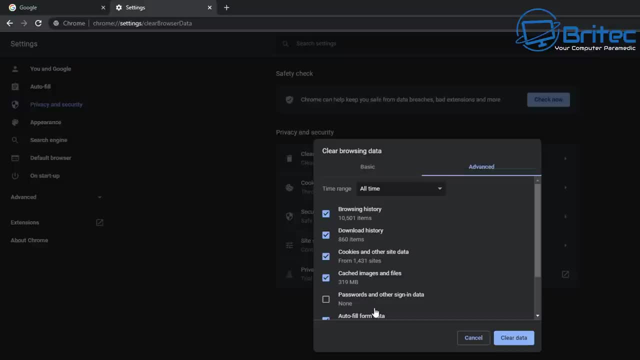 thinking your signing information will be safe. It won't be if you leave in cookies and other site data. It's important that you understand that all these signing data will be removed, like your sign in and password information. So if you don't have them saved, then 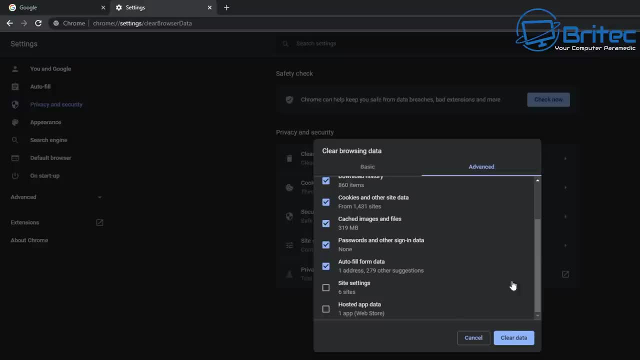 they will be removed when you run this cleaner. It's important that you do this on a regular basis to remove all of the data from your computer, and this will remove any sort of junk that's stored in temporary internet files and other locations like that. You've got the time gap here range. 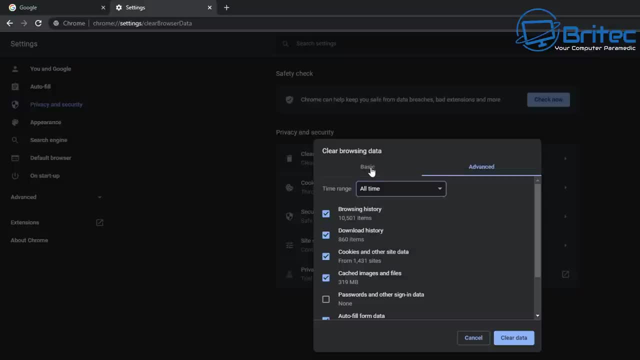 which is the last hour, 24 hours, seven days, four weeks and in all time. It's always best to do all time. It will completely remove everything from your browsing history. Sometimes it's going to help speed up a little bit more page loading times. 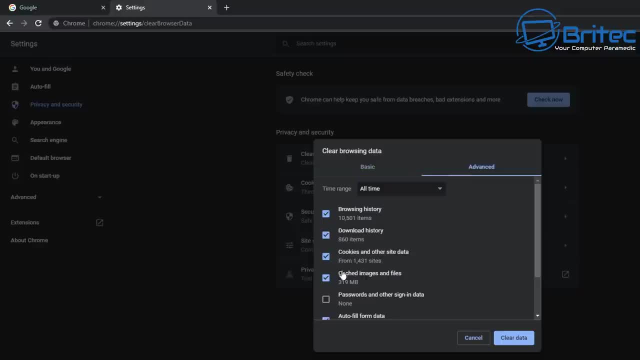 after you've cleaned this, Especially if you've got a lot of junk inside here and it ends up in gigabytes in size. I see people not running this on their computer on a regular basis and it does actually hinder performance with your browser. So I like to run this on a regular basis. 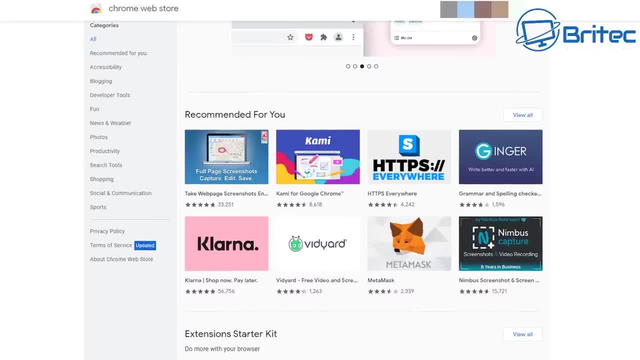 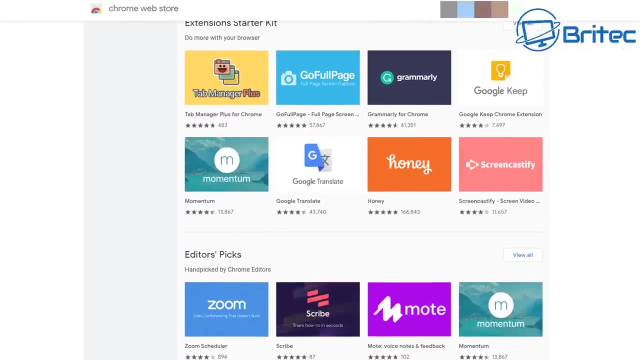 Next up. we're talking about browser extensions. Are they safe? Should you use them? So many people use browser extensions and, to be honest, some browser extensions require access to almost everything that you browse on the internet. They can sometimes see sites that you've visited and 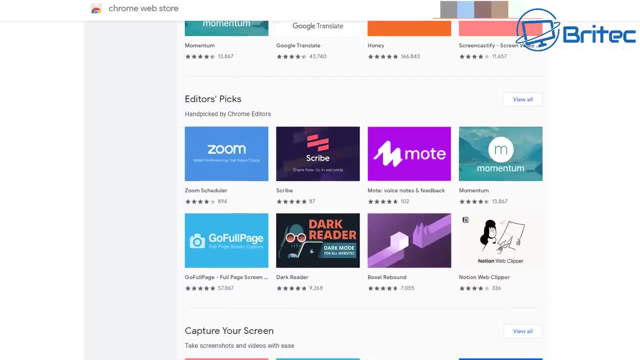 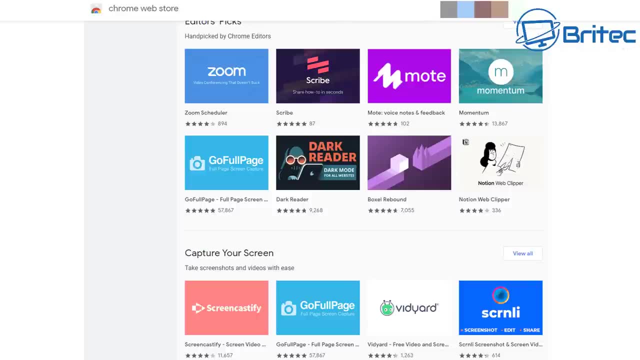 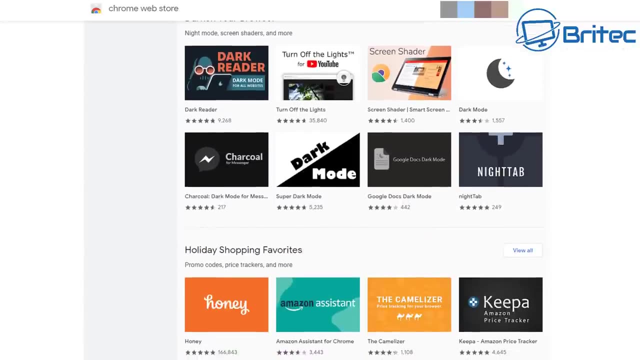 also view your keystrokes and even passwords. So not every browser extension is safe, and some may be malicious, So be careful which ones you install on your system. try to keep your browser as default as possible without the need for all of these extensions, because some of these are. 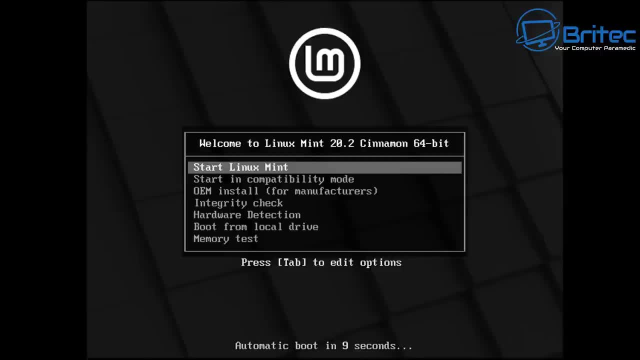 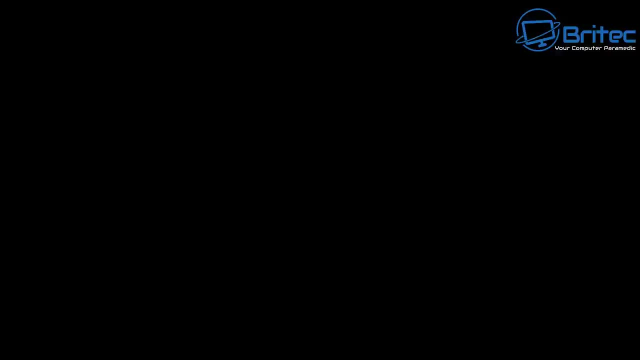 harvesting data from you, for which ones you install Next up. if you want to do banking online, try downloading a Linux distro and create a bootable USB flash drive with that distro and then basically, you could just put that into the computer and boot up to it. This is not going to install on your computer what it's going. 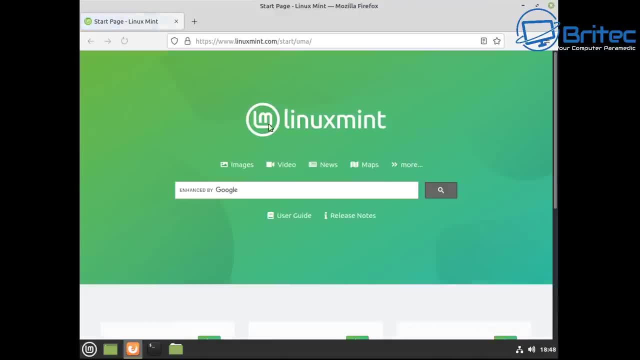 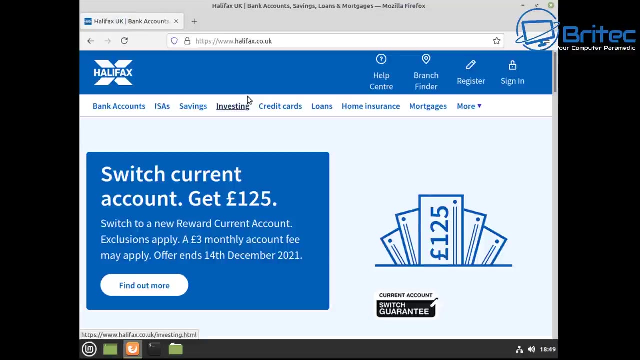 to do is boot up what we call a live environment, and you can see here I can access the internet and basically searched for my bank of my choice and then log in and basically do my banking through this method here. What is the benefit of doing it this way? Well, it means that nothing is. 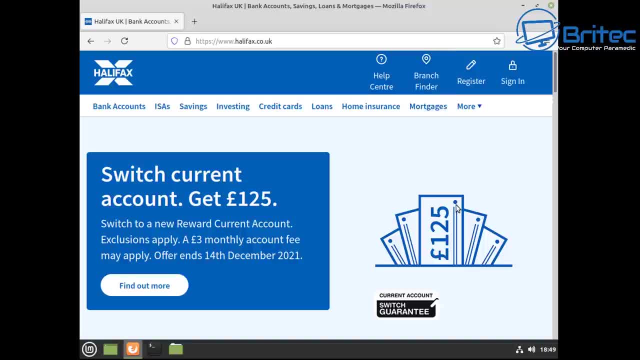 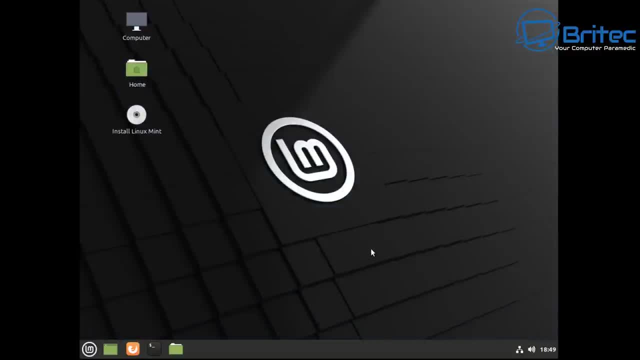 running in the background. that means any malware or any other stuff that may be on your computer or your browser may be infected. it's not going to matter, because we're booting up to a live environment where there's nothing running in this sort of environment, which makes it much more safer. 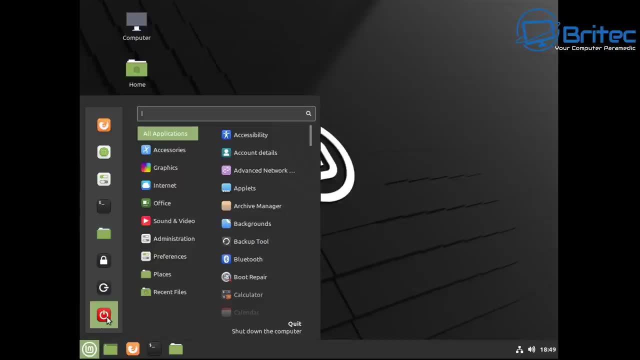 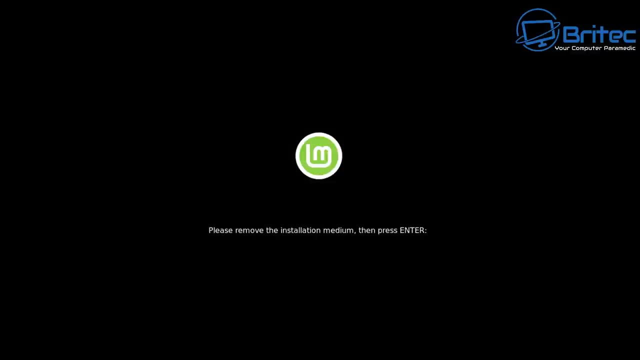 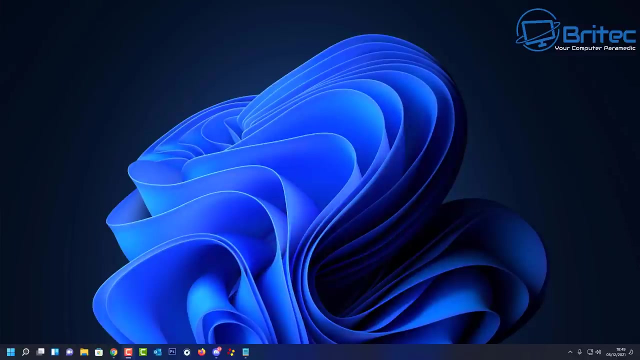 to do online banking. you're not installing Linux on your system. when you shut down, it will go back to your Windows operating system. this is the safest way to do online banking, in my opinion. it means that you won't have any sort of malicious code or anything like that running in the background. 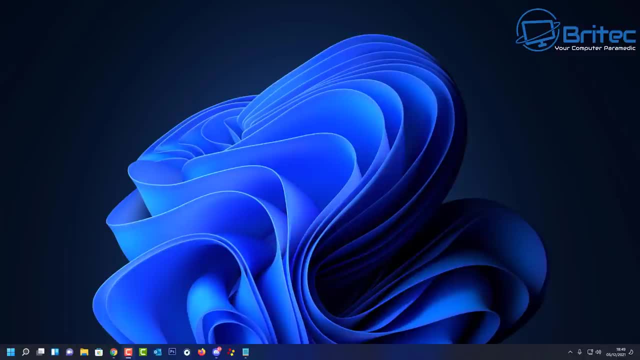 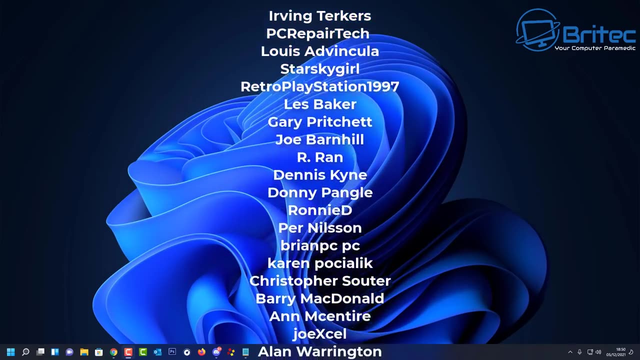 which could basically steal your details when you log on to your bank. Anyway, that's going to be about it for this video. hope this video helps you out. my name has been Brian from britechcomputerscouk. just want to say a big thank you to all of you for watching this video and I'll see you next time. 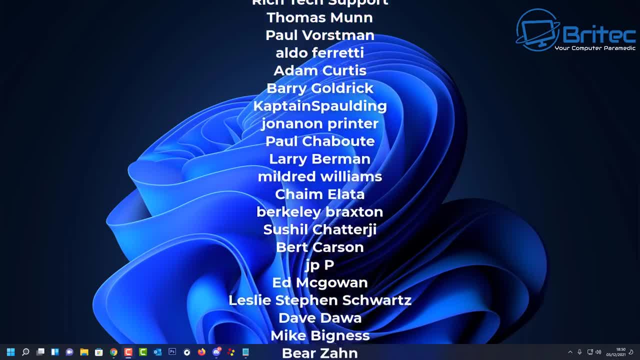 big shout out to all my YouTube members who join my YouTube members group. your names are rolling up on the screen right now and I shall see you again for another video real soon. thanks again for watching. bye for now.